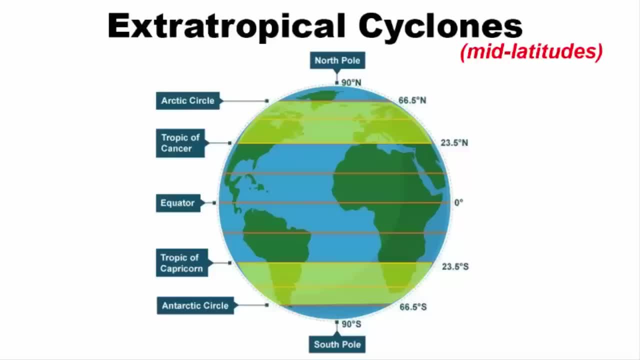 This region is called the mid-lattitudes. That is why extra-tropical cyclones are sometimes called mid-latitude cyclones, And some part of the cyclone even touches the high latitudes. Generally, in between 25 and 35 degrees north and south latitude, you will find the subtropical. 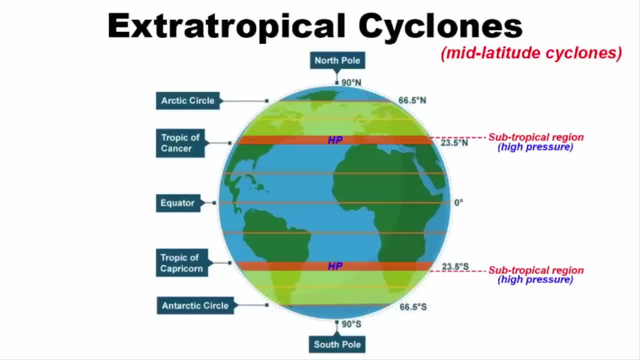 region, which is a high-pressure belt, And it is also a transition zone from tropics to temperate region. And then, in between 50 degree and 70 degree north and south latitude, you will find the subpolar low, which is a low pressure belt, And in between 50 degree and 70 degree north and 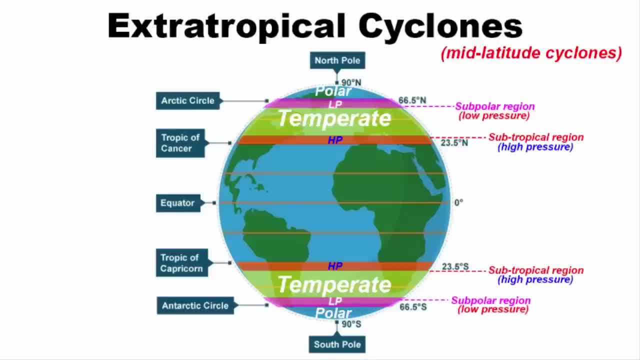 south latitude, you will find the subtropical low, which is a low pressure belt. And this is a low pressure belt and it is a transition zone from the temperate to polar region In between. the westerly winds are very active in this region and they flow from the west. 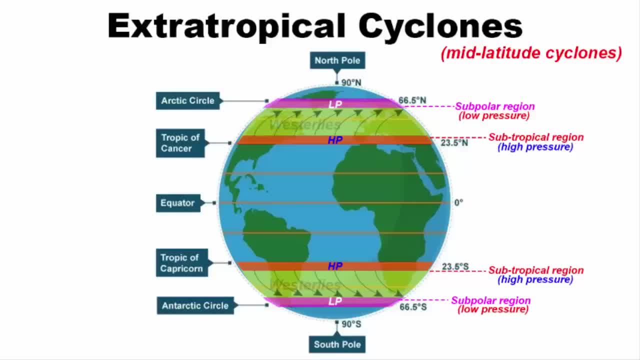 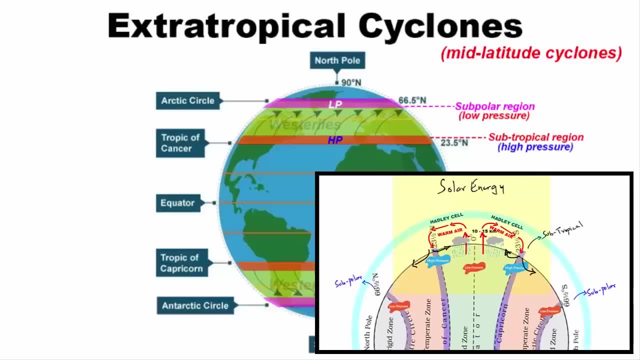 towards the east. If you are interested to know how these high pressure and low pressure belts are formed at different latitudes, I have a separate video on it. again, the link will be available in the description and also at the end of this video. 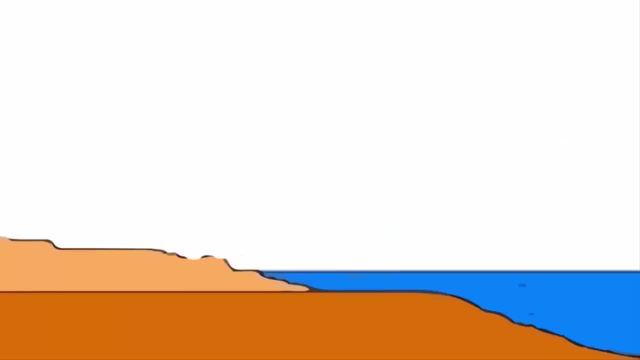 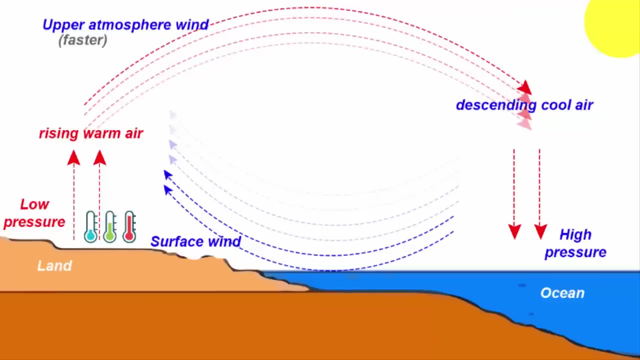 Now we will see how the extra-tropical cyclones are formed. Try to understand this. wind circulation is the main reason that creates any kind of cyclone And, depending on temperature, winds propagate between the surface and the upper atmosphere. And always remember upper atmosphere winds are faster than surface winds because friction. 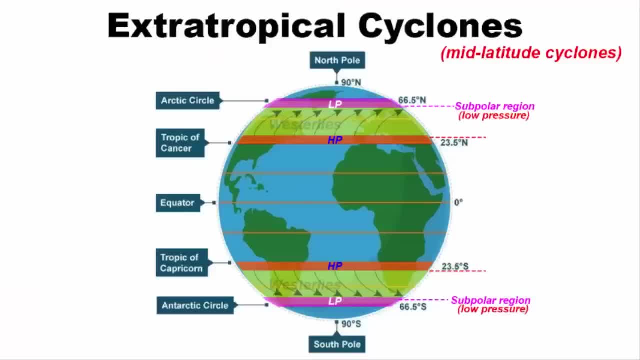 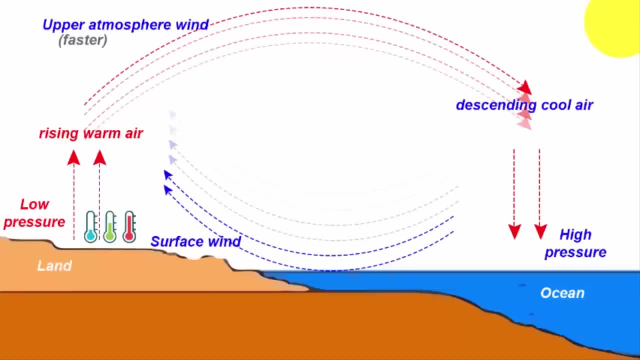 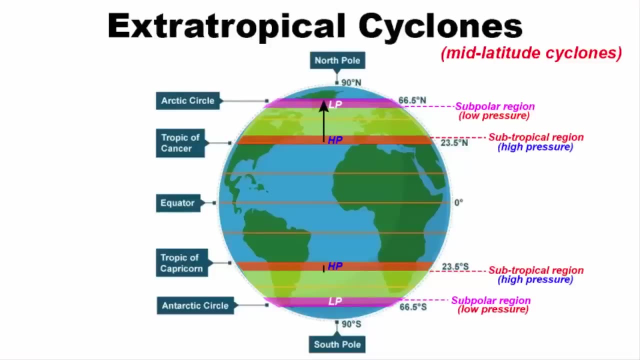 slows surface winds. We have already learnt that the subtropical region is a high pressure belt and then the subpolar region is a low pressure zone. We also know that air moves from high pressure areas to low pressure areas. That means there will be air movement from subtropical high to subpolar low at the surface. 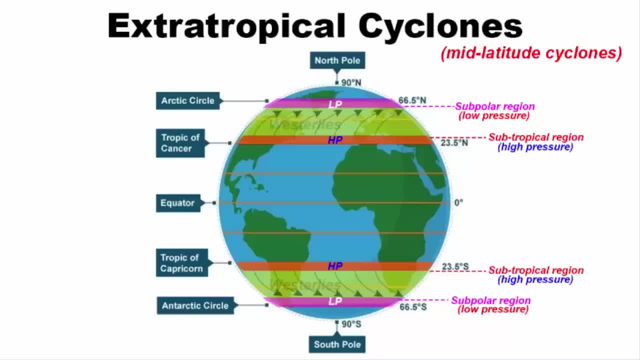 level. Due to Coriolis effect, this wind gets deflected to the right, and that's what lead to the prevailing westerly winds. And then there are winds that occur high in the atmosphere, somewhere between 12-15 kilometres above the ground. 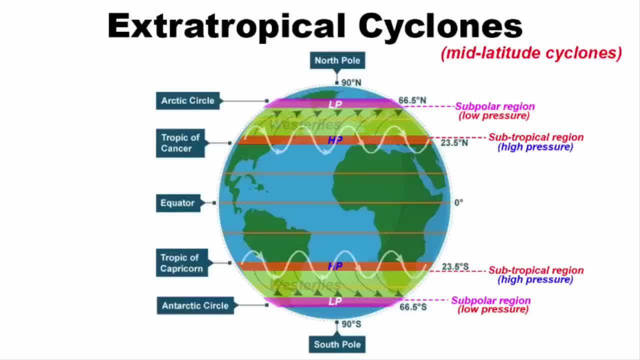 These are called the subtropical jet stream. They flow from west to east And it is also one of the strongest winds on earth. The speed of this wind may go up. It may go up to as much as 500 kilometres per hour. The subtropical jet stream sits between the Hadley and Ferrell cell And, keep in mind, here the wind descends. That's what creates the high pressure zone. There's another jet stream that sits at the subpolar region, In between the Ferrell cell and Polar cell. 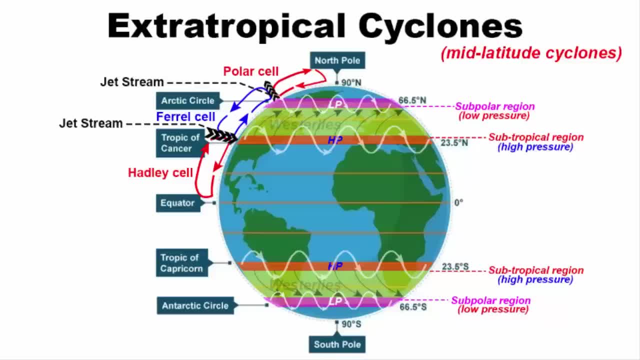 And we know, here the air rises. That is why this region is a low pressure zone. That means jet streams form in between cold polar air and warm tropical air of both the hemisphere. Even the jet stream gets deflected by the Coriolis effect. 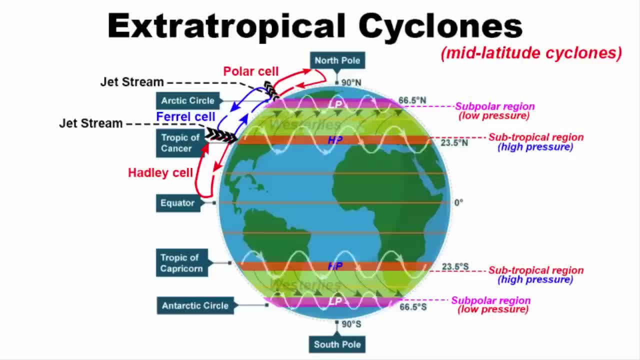 But not much, Very little. Jet streams does not maintain a straight flow from west to east. It rather moves like a snake and dips to the south or rises to the north. So far we know that both the wind at the surface and at the upper atmosphere are subjected. 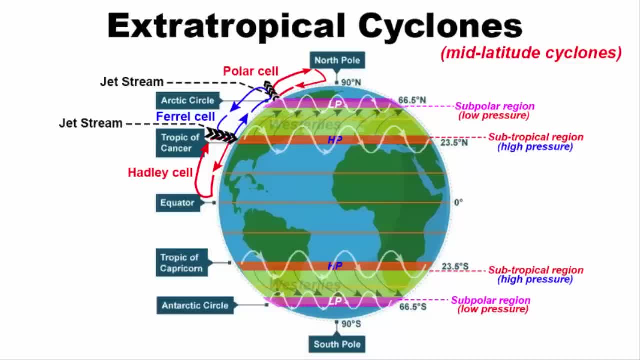 to deflection due to Coriolis force. And now begins the main explanation for the extra-tropical cyclone. When air descends at the surface, the wind is subjected to a deflection due to Coriolis force. And now begins the main explanation for the extra-tropical cyclone. 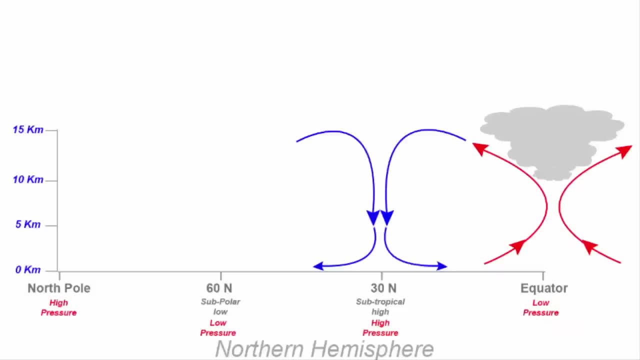 And, as you see, the causer is torrential and so near to down. enjoying warming. wszystko in the surface can give great damage And, by the way, these are warm air. As we go more and more towards the polar region, temperature drops. 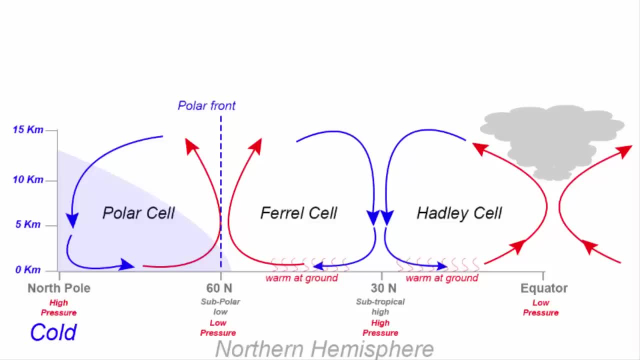 It gets cold Because cold air is also moving from the poles towards the warmer region. Since cold air is dense and heavy, it usually flows nearer to the ground, making the nearby environment also cold. Thismon analysts estimated that the temperature drops from 50 to 150 degrees Celsius. 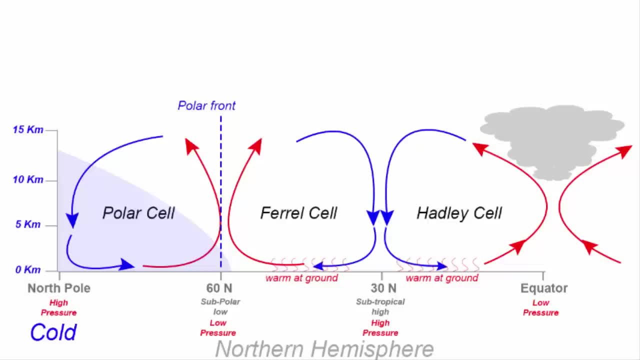 But then the entire polar region is cold. so air is cold everywhere, both at the surface below 9 to 120 degrees, as well as in the upper atmosphere. I'll try and illustrate it in the best possible way. please try to follow up. 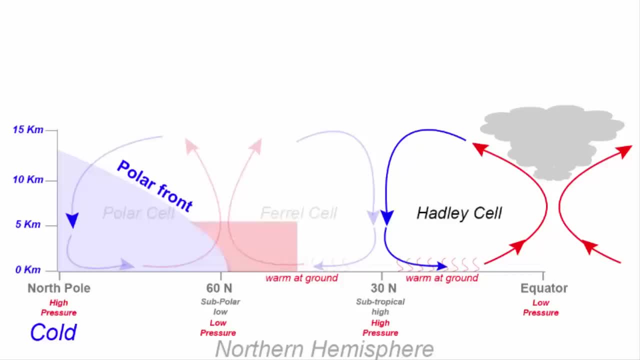 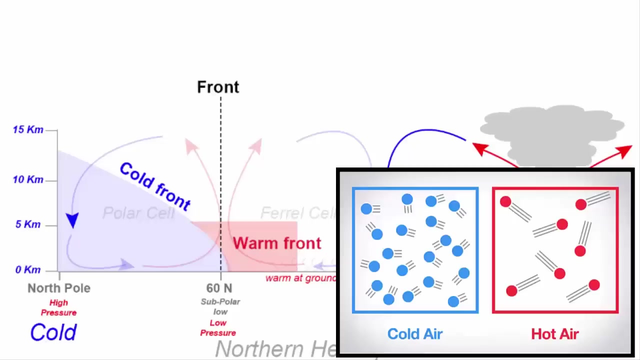 So there has to be a boundary where the cold and warm air meets. That boundary is called a front. That boundary is found near the sub-polar region. So naturally this becomes the cold front and this becomes the warm front, Since the warm air is light and it expands. on the other hand, cold air is dense and heavy. 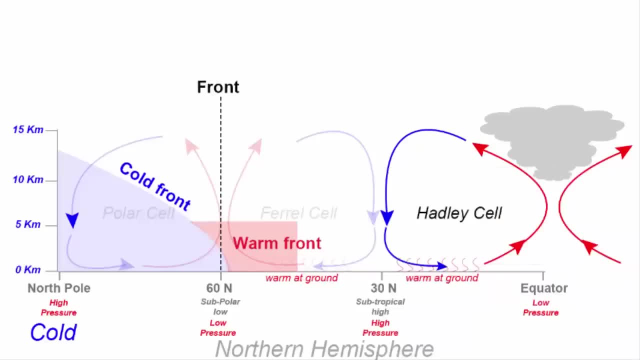 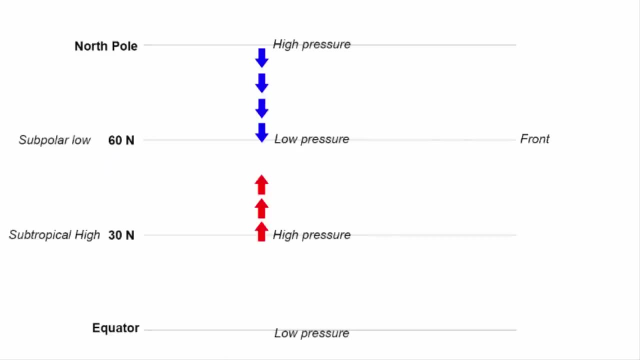 I'll only show the northern hemisphere Once you understand. the same principle applies to the southern hemisphere too. When warm air approaches the cold air from the south, it gets slightly deflected towards right due to Coriolis effect. This is what becomes the prevailing westerly winds. 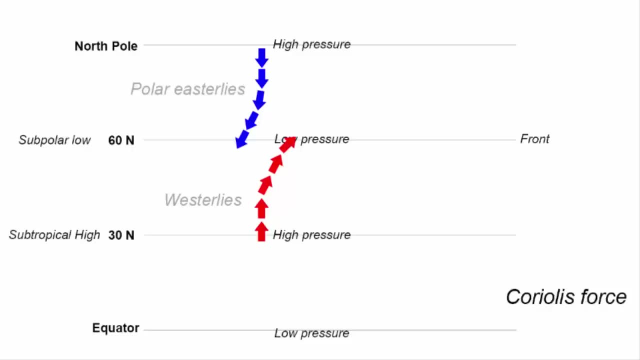 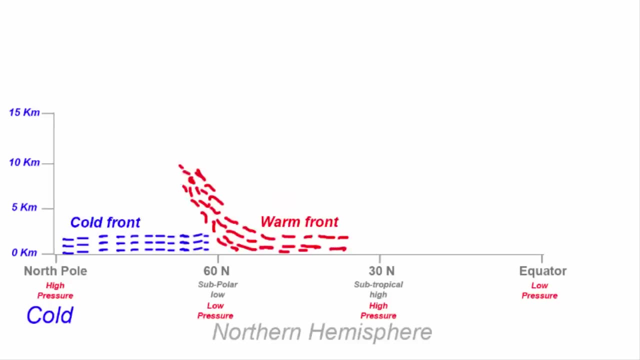 Similarly, when cold air from north pole approaches south, it gets slightly deflected to left As the warm air approaches the cold front. since the cold air is dense and heavy, it pushes the warm air upward. This region is usually called the cold front.